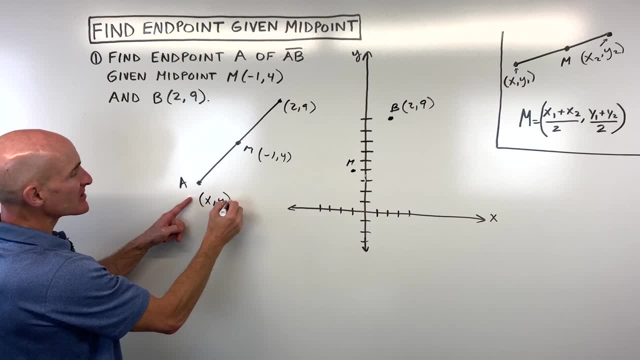 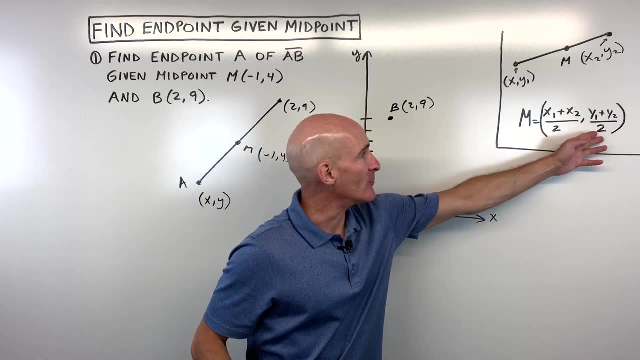 point A, which is what we're trying to solve for Let's just call it x comma y, because we don't know the x-quad and the y-coordinate. Now, when you find the midpoint, it's like finding an average, Like you add the x-coordinates and divide by 2, that's how you find the. 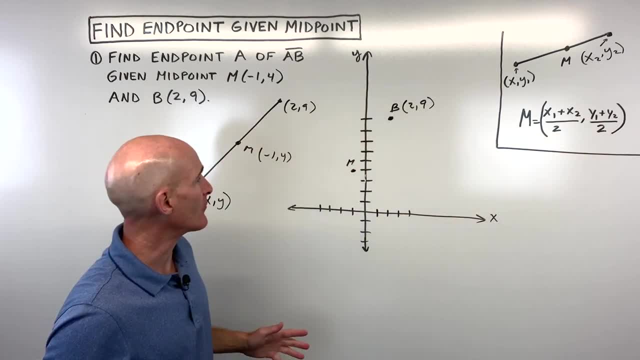 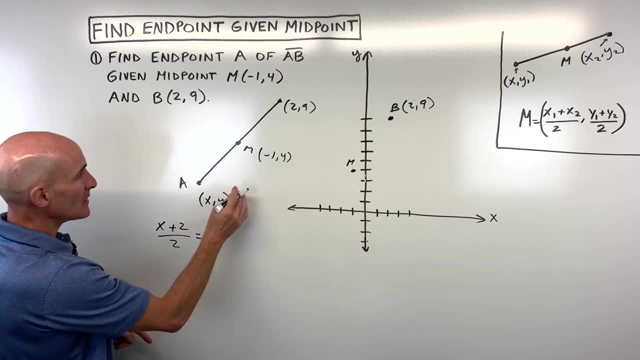 middle, and then you add the y-coordinates and divide by 2.. So just like an average. So what we're going to do is we're going to say x plus 2 divided by 2 equals the x-coordinate of the midpoint, And we're going to do the same thing for the y's. 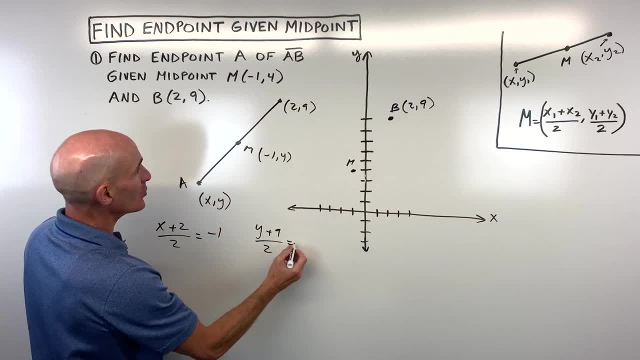 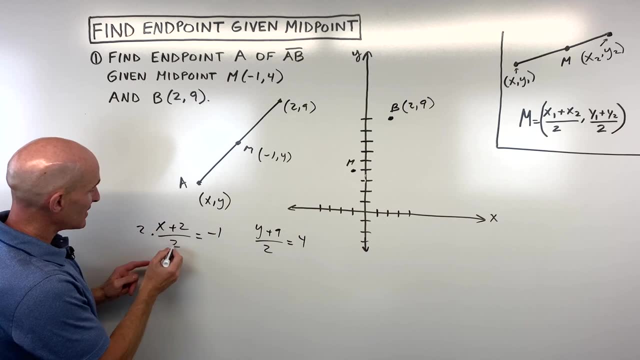 y plus 9, divided by 2, equals the y-coordinate of the midpoint. Okay, now we're going to solve these two equations. We're going to multiply both sides by 2.. Instead of dividing by 2, we're going to do the opposite: Multiply both sides by 2.. So now we have. 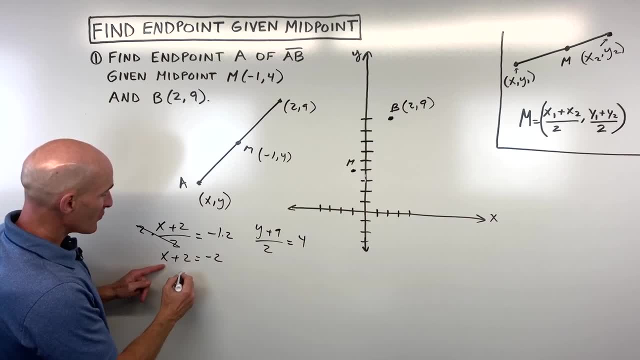 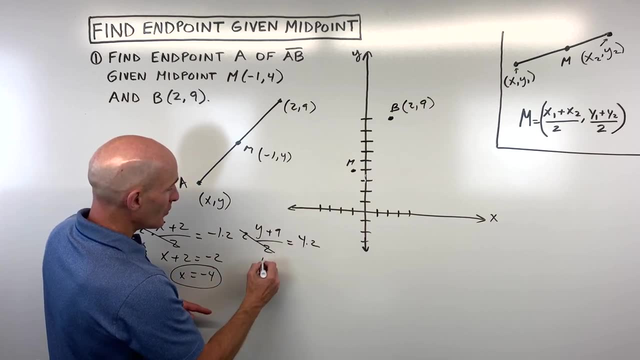 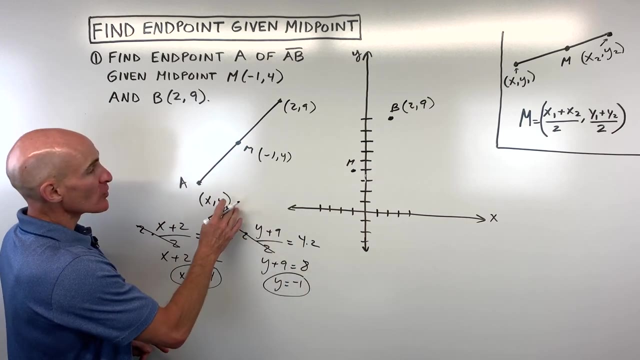 x plus 2 equals negative 2. And if we subtract 2 from both sides, you can see that x equals negative 4. Over here, if we multiply both sides by 2, we get y plus 9 equals 8. And if we subtract 9 from both sides, we get y equals negative 1. So the 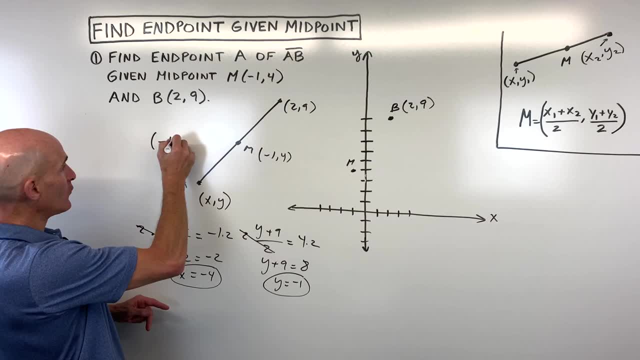 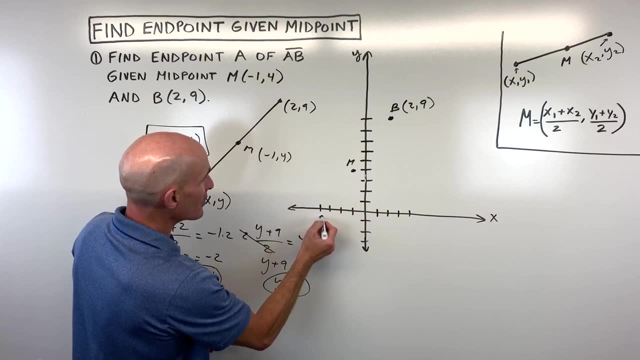 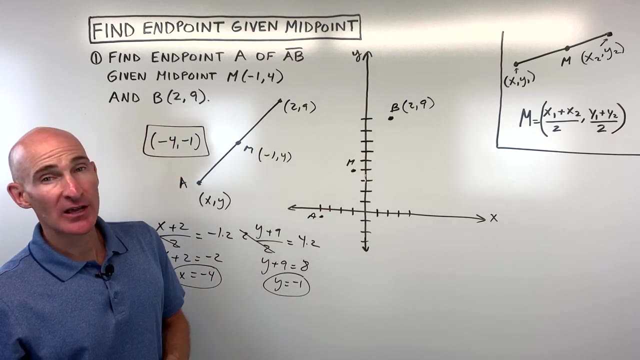 coordinates of our point here. a is going to be at negative 4,, negative 1, and if we plot that you can see this is left 4, down 1 right here and you can see that the midpoint is halfway between point A and point B. Now I was telling. 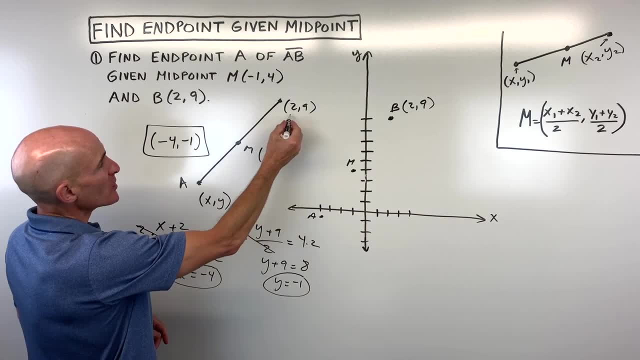 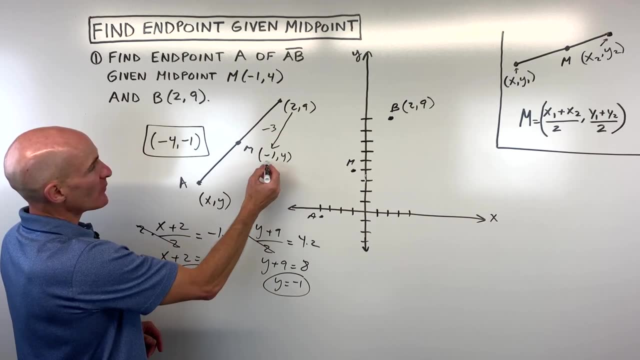 you. there's a shortcut method for doing this, and let me see if I can show you this. So what you would do is you'd say: hmm, how am I getting from 2 to negative 1?? Well, you can see, I'm subtracting 3. so if I do that same thing, if I subtract- 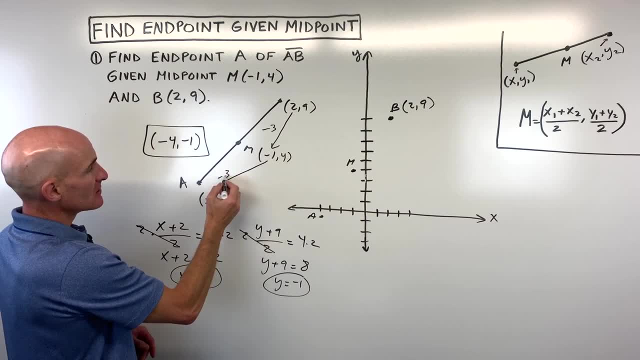 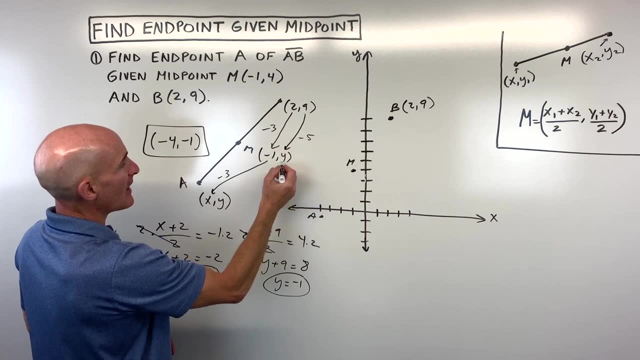 3, again negative. 1 minus 3 gives us negative 4, right, Let's do the same thing for the Y. So how am I getting from 9 to 4? I'm subtracting 5. so if I subtract 5, 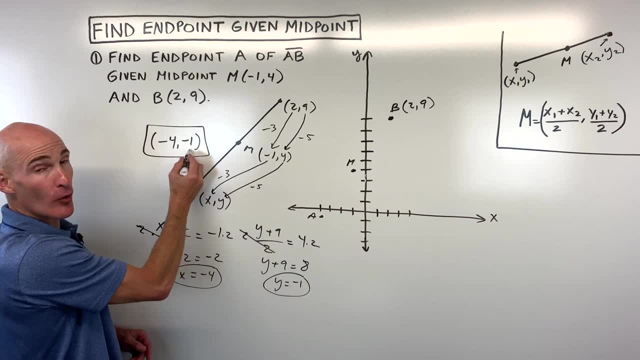 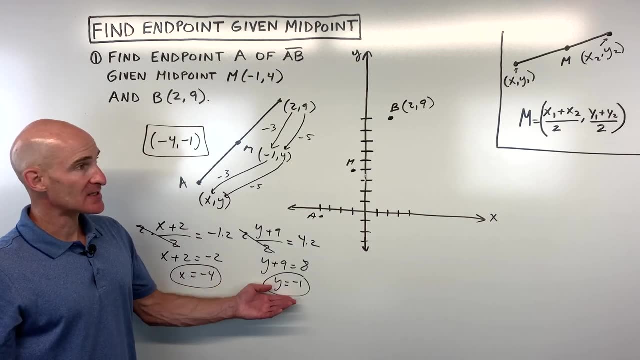 again, what's 4 minus 5? Negative 1.. Now this is good for taking like a standardized test, but usually when you're doing it like on a test in your class, your teacher is going to want to see the use of the midpoint formula here. 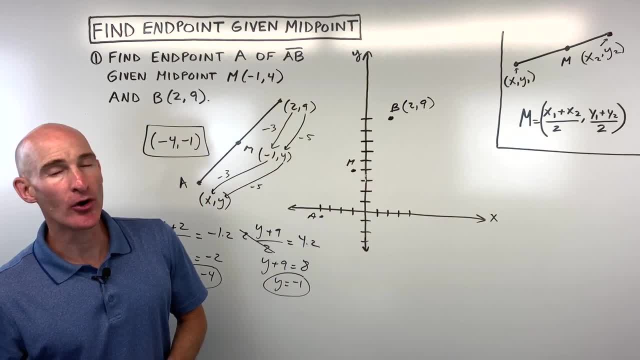 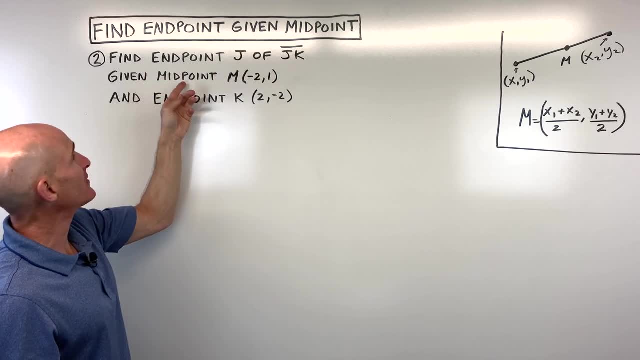 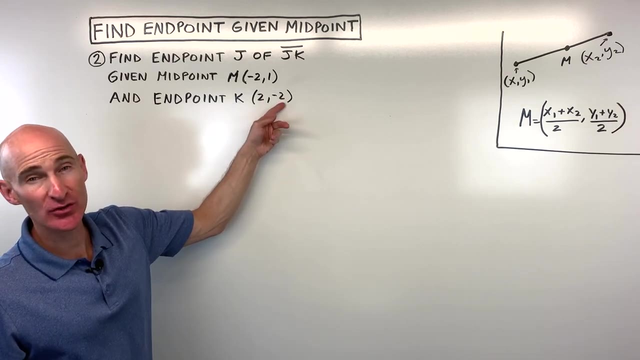 So let's take a look at another example. see if you can do this one on your own. Okay, For number two, we have find endpoint J of segment JK, given that the midpoint M is at negative 2, 1 and the other endpoint, K, is at the point 2, negative 2.. 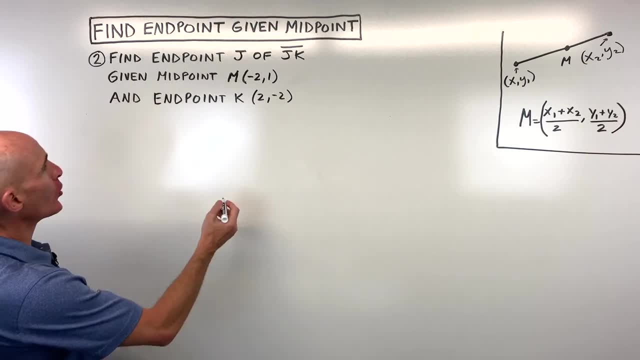 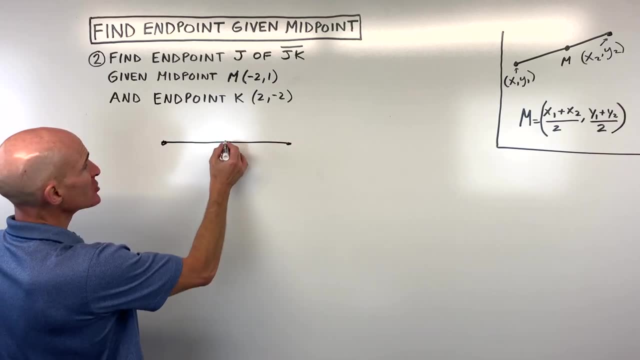 How would you do that one? See, if you can pause the video, try this one on your own. The way I like to do it is just draw a segment. It doesn't have to be like a perfect graph, like in a XY coordinate plane. You can just draw something just. 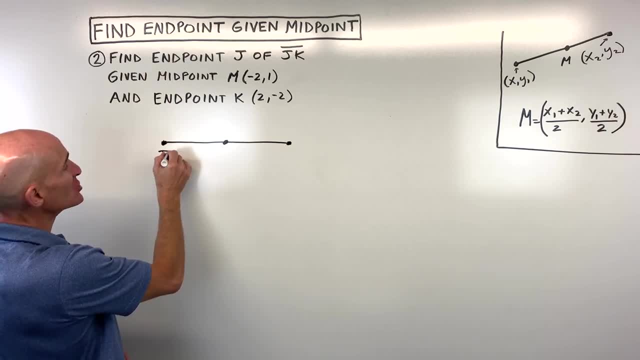 kind of back of the envelope style here, where we have endpoint J, endpoint K and the midpoint M. So we have endpoint here in the middle, that's negative 2, 1.. J, we don't know, so let's call that X, Y and K. we do know which is at 2, negative 2.. 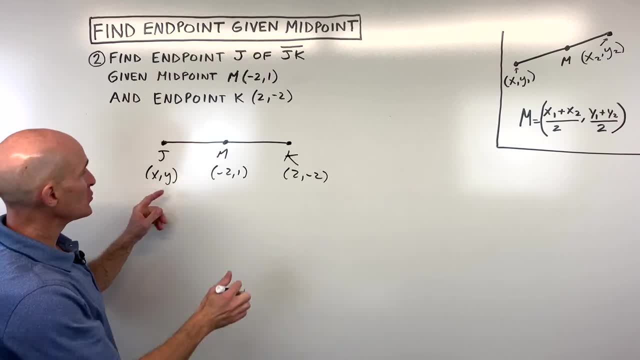 So let's do the formal method first. So what I would do is I would average the two endpoints to get the midpoint. So I'm going to say X plus 2. so add the two X coordinates together and divide by 2, and that equals the X coordinate of the. 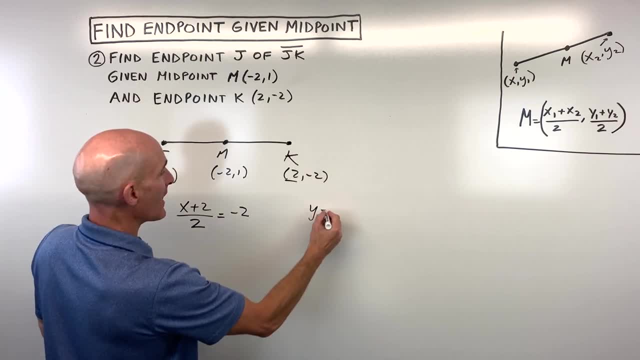 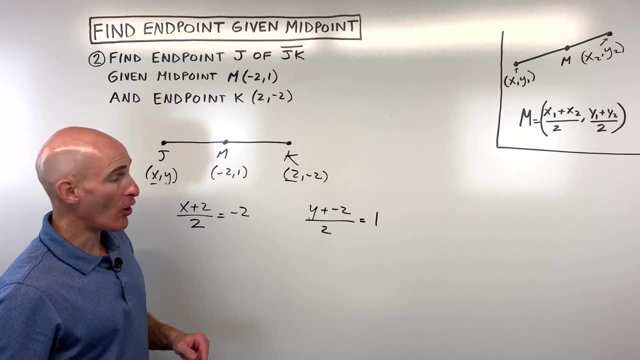 midpoint. Let's do the same thing for the Y. So we're going to say Y plus negative 2, divided by 2, equals the Y coordinate of the midpoint. Okay, now all we have to do is solve. So I'm going to, instead of dividing by 2, I'm going to. 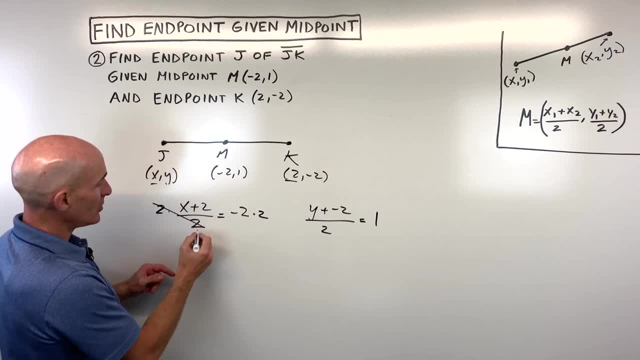 multiply both sides by 2.. That way these cancel. We've got X plus 2 equals negative 4.. If I subtract 2 from both sides, we get X equals negative 6 and over here. if I multiply both sides by 2, the 2's cancel. We get Y plus usingacción y-2. 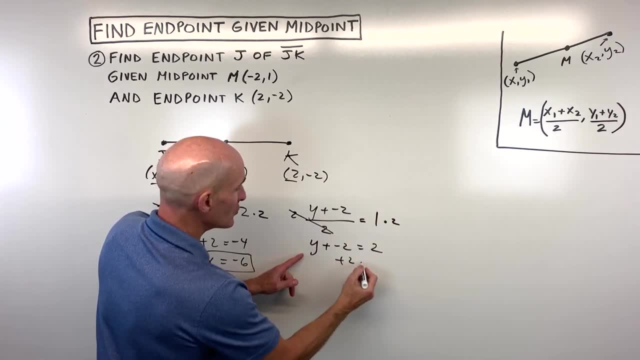 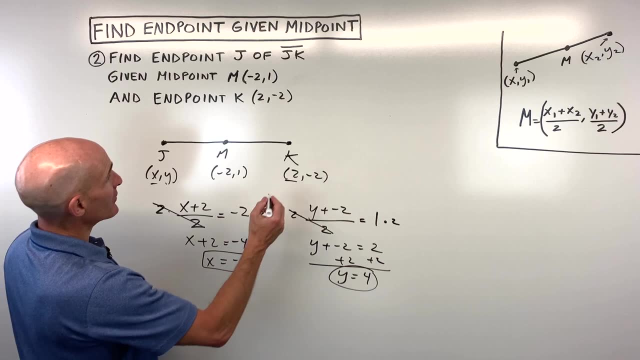 plus negative 2 equals 2, and if I add 2 to both sides, you can see that y is coming out to 4, and so that's the end point. over here it's going to be at the point, so j is at negative 6. 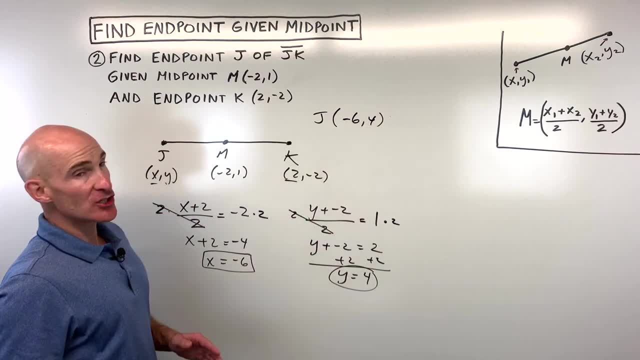 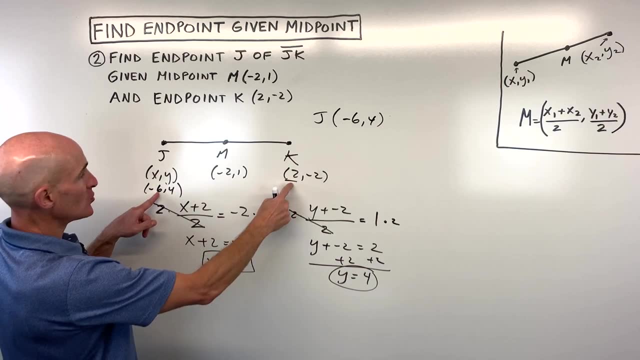 comma 4.. Now another way to check your work is to go ahead and look at negative 6- 4. you could say negative 6 plus 2 is negative. 4 divided by 2 is negative 2. that checks out 4 plus negative 2 is.